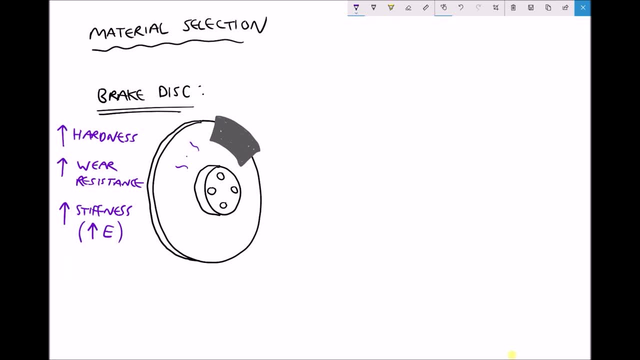 elasticity. It's a little counter-intuitive, but high elastic modulus means low elasticity, and high elastic modulus means high stiffness, which is the inverse of elasticity. Now, the final property that we're going to consider is thermal expansion. We're going to want low thermal expansion. Now, the reason for this is because, as this brake disc 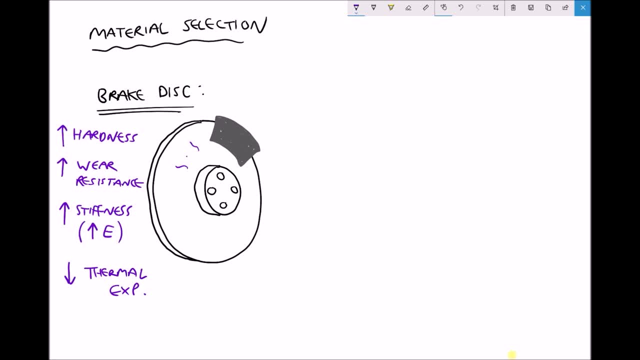 becomes hot. the last thing we want is for it to expand, because if it expands it may decrease the distance between our brake pads. If the distance between the brake pads changes, we may find that the brake disc pictured here in white would actually rub against the brake pad pictured. 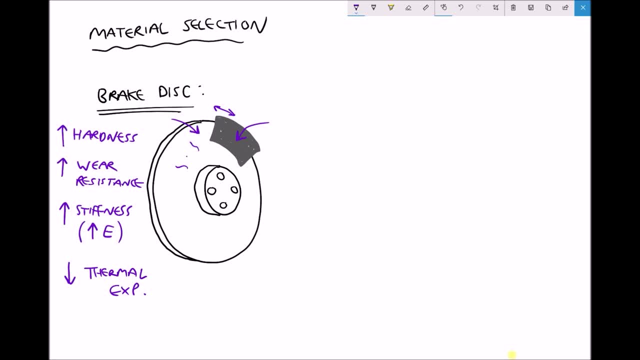 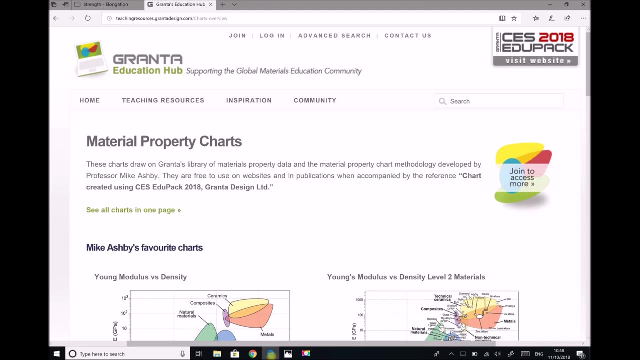 here in grey. So ideally, we want a low coefficient of thermal expansion to prevent this from happening when the brake disc becomes hot. So, first of all, let's look at hardness and wear resistance And, once again, the chart that we're going to use was created using the CES EduPak 2018 provided. 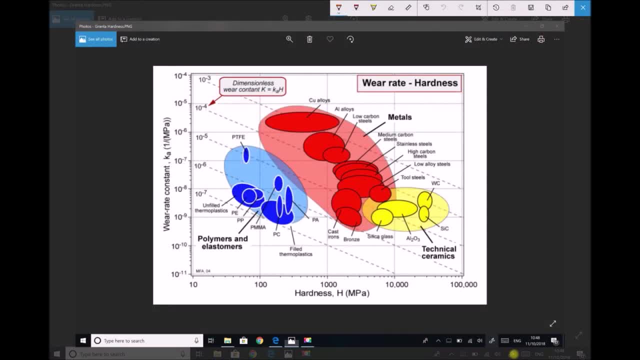 by Granter Design Limited, and here's the image of the chart that we're going to use. So, first of all, if we look at our two axes, on the y-axis we have wear rate, and this wear rate is a measure of how much material is lost during a given process under an applied stress. 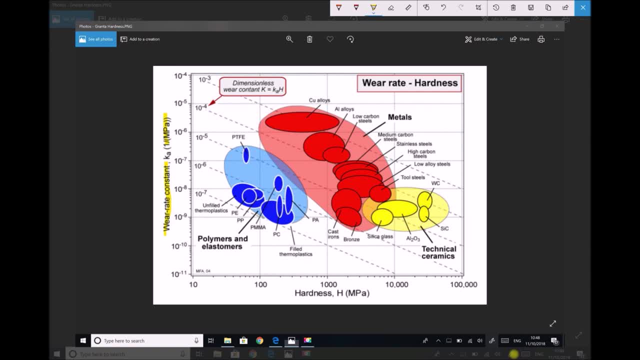 So we have two surfaces being pushed together with a particular stress and, as a result of movement between those surfaces, we're going to lose material. So this information will have been obtained through extensive testing. On the other axis, we have our hardness, and the hardness of the material is its 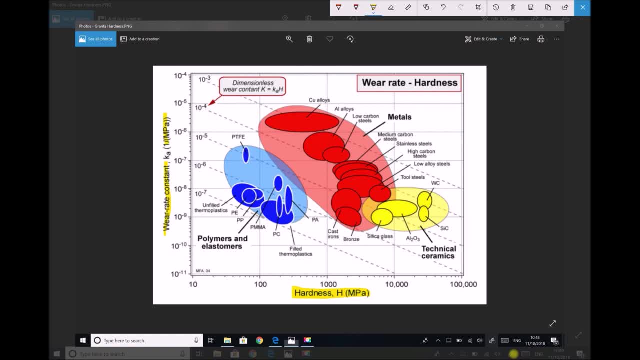 resistance to scratching and indentation. Now, once again, if we look at our scales, these are logarithmic scales. so we see, on our x-axis we go from 10 to 100 to a thousand- it's not a linear scale. and on our wear rate we have materials which 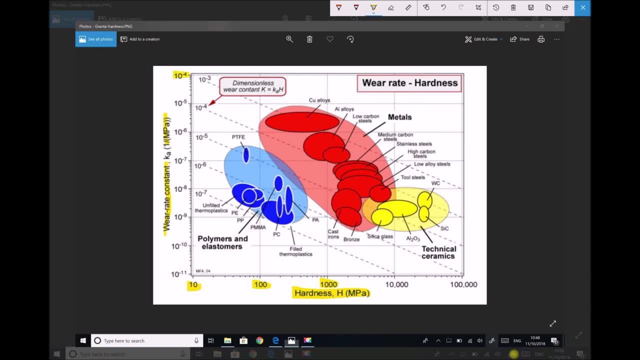 wear readily with wear rate constants of 10 to the minus 4, and we see that number decreasing. So essentially we want the materials with the lower wear rate, the materials that are less likely to wear. So we're looking for high hardness, low. 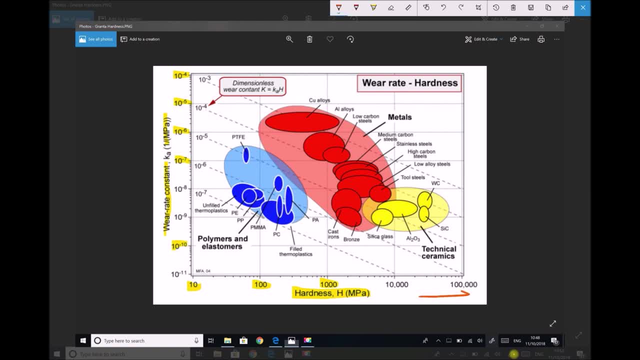 wear rate. Well, high hardness is going to be on the right hand side of our x-axis, and low wear rate is going to be on the right hand side of our x-axis and low wear rate is going to be near the bottom of our y-axis. As you would expect, the harder the material, the 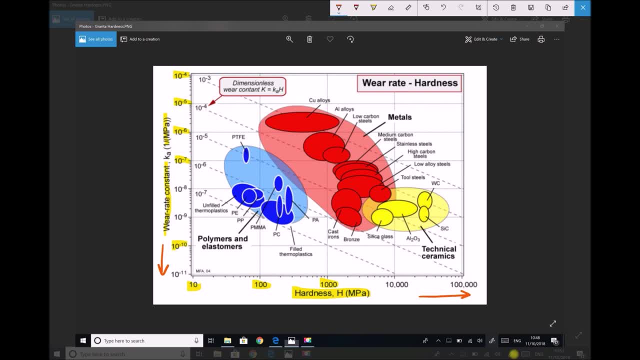 less readily it's likely to wear. Now we're going to consider two different materials during this analysis. One of the materials we're going to consider is cast iron, and the other material that we're going to consider is silicon carbide. Both of these materials are commonly used in brake discs. Cast irons. 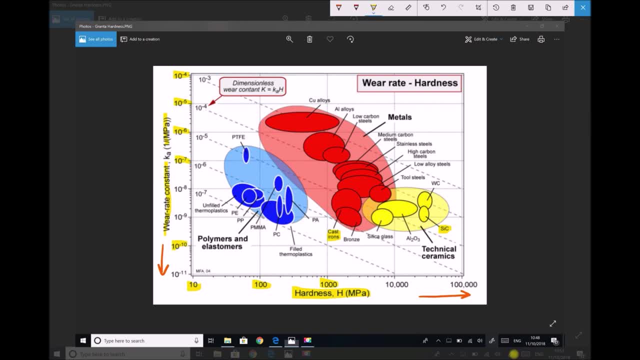 are commonly used in brake discs, whereas silicon carbide tends to be used in performance vehicles. So we're going to analyze each of those Now. what we notice about each of those materials is they're very well matched in terms of wear rate. They're both sitting at around 10 to the minus 9 on that axis, Where these two 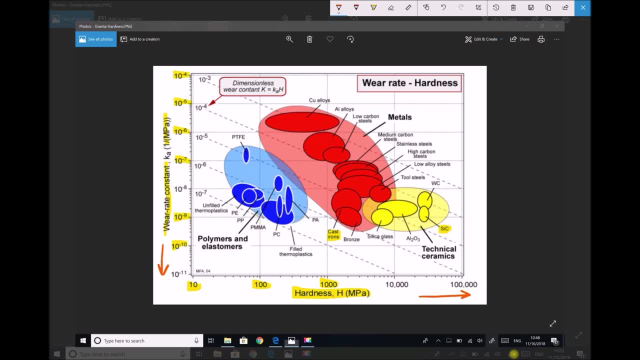 materials differ is in terms of hardness, and we see cast irons sitting at a hardness of around 2000.. But if we look at our silicon carbide, then we'll have a we have hardnesses of around 30,000.. Because we have that logarithmic scale. 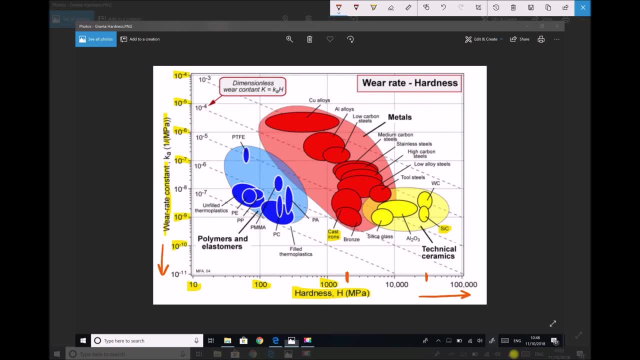 that small distance represents a large difference in terms of hardness. So 2,000 for cast irons, whereas silicon carbide somewhere in the order of 30,000 megapascals for the hardness, So comparable in terms of wear resistance. 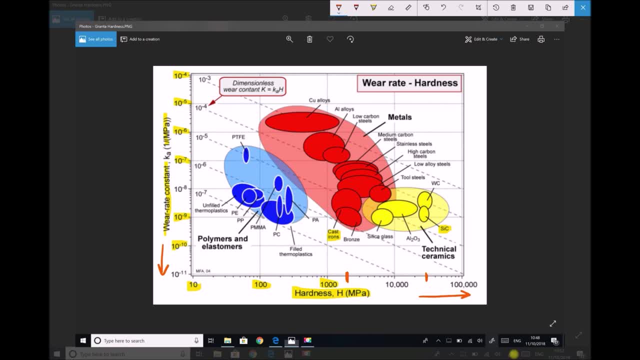 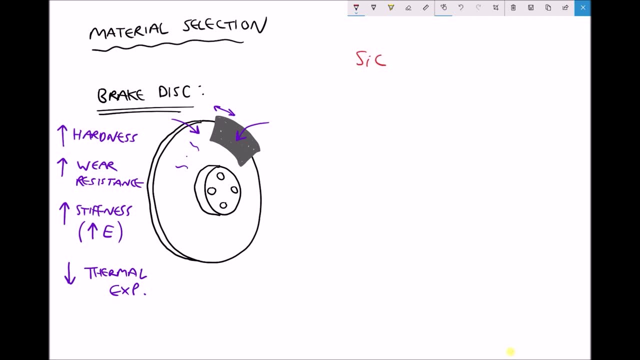 but silicon carbide appearing to be better for hardness. So we're shortlisting silicon carbide and we're shortlisting cast iron, And we've found that silicon carbide has better hardness, but we've found that their wear resistance is comparable. So at the moment we have one positive for silicon carbide. 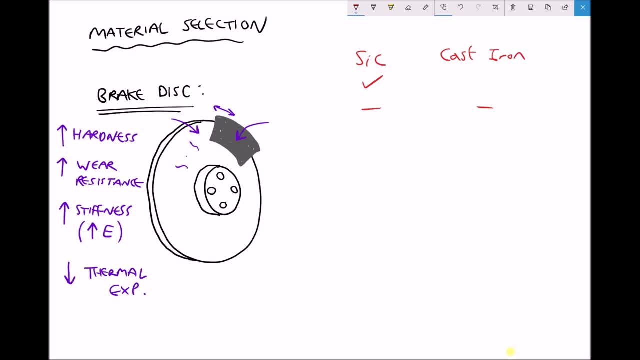 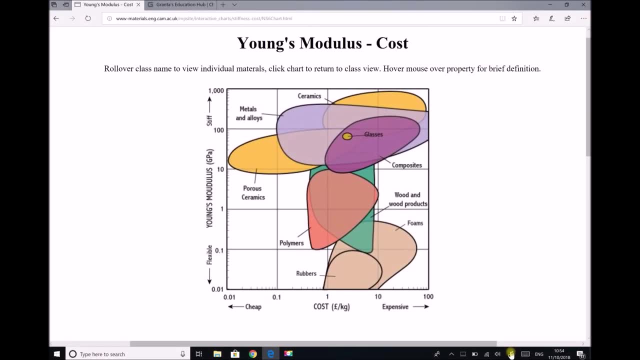 and a positive for both silicon and cast iron in terms of their wear resistance. Let's look at stiffness and thermal expansion next. So once again we have a chart from materialsengcamacuk And again I'm going to provide links under these images on the study platform. 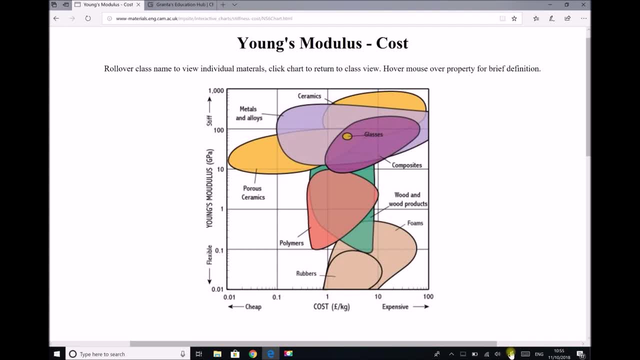 We need to look at two materials. We need to look at the ceramic material- silicon carbide- and we need to look at the metal, cast iron. So let's highlight our metals group. first of all, And we can see here, the cast iron has a stiffness or a Young's modulus. 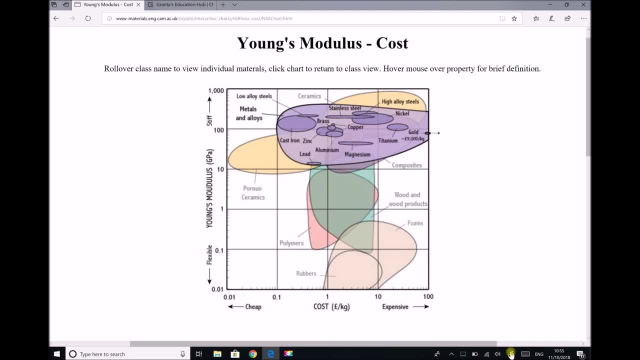 between 1.5 and 1.5 mm. So that's the cast iron. So we've got our silicon carbides here. We're looking at what they look like when they're balanced. So on the silicon carbide, you can see how they are. 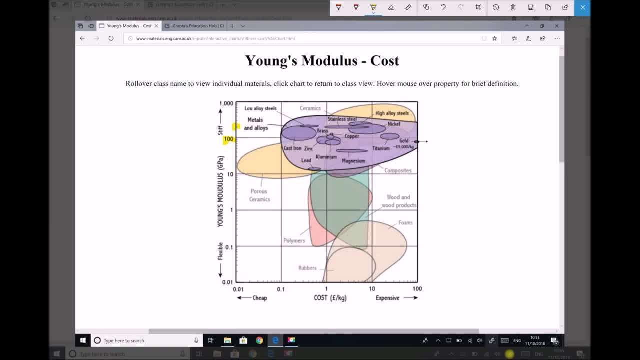 It's about one and a half gigapascals And this is the casting heat. It's about one gigapascals. They're about 100.. It's about 100 gigapascals for the cast iron and that's about 100 gigapascals for the cast iron. 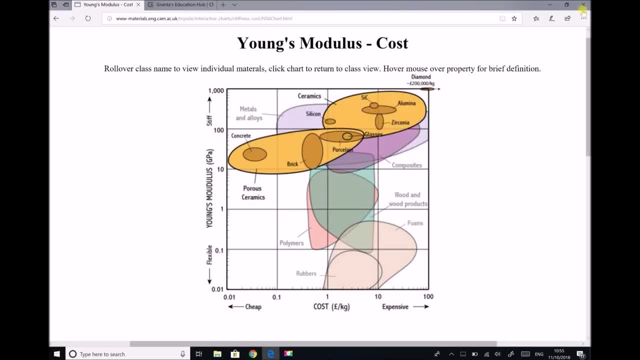 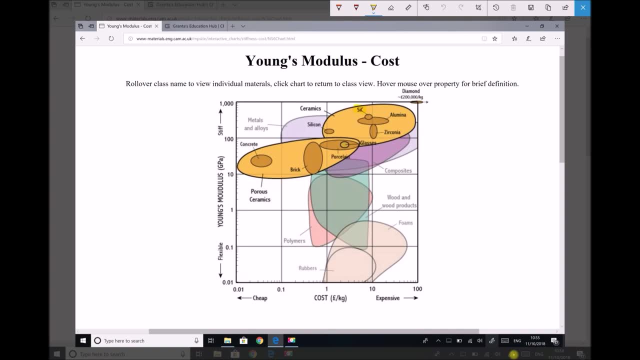 And, what's more important, they are about 100 gigapascals here and 100 gigapascals here. So 100 gigapascals here. carbide here, and this time silicon. carbide has an elastic modulus somewhere in the order of 400. 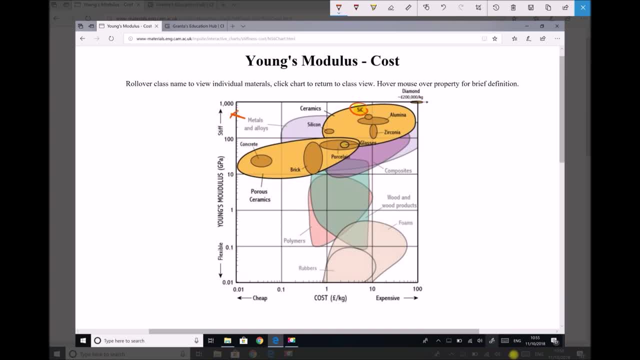 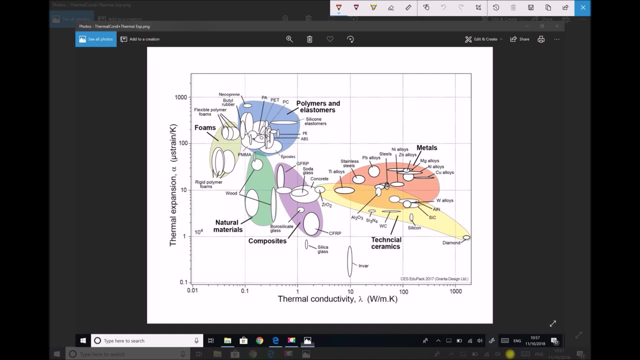 gigapascals. so once again, in terms of stiffness, the silicon carbide outperforms the cast iron. we have one last property to look at: thermal expansion, and once again we have a chart that's been produced using the granta ces edu pack- this time the 2017 version, and the axis that we're interested in this time is our y-axis for thermal. 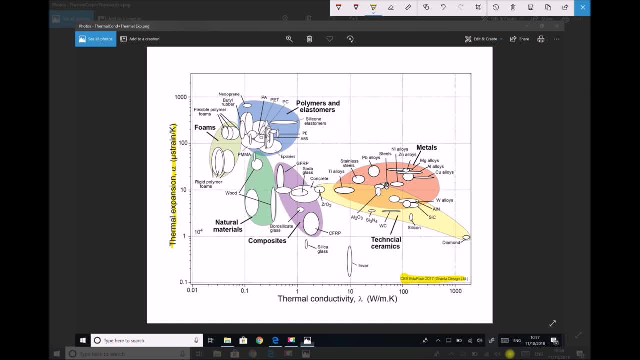 expansion. we need to consider two materials. we need to consider cast iron and whilst cast iron isn't on here, we would expect the thermal expansion of cast iron to be a little bit be very similar to high carbon steels. Cast iron, in effect, is a carbon steel with a percentage carbon. 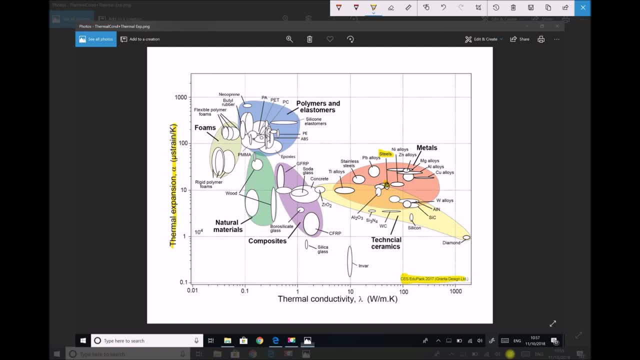 above two percent. The other material that we're considering is silicon carbide. here in the technical ceramics section. Now recall that we're looking for a material with a low thermal expansion. We don't want the brake disc to expand upon heating, so we have cast iron with a coefficient. 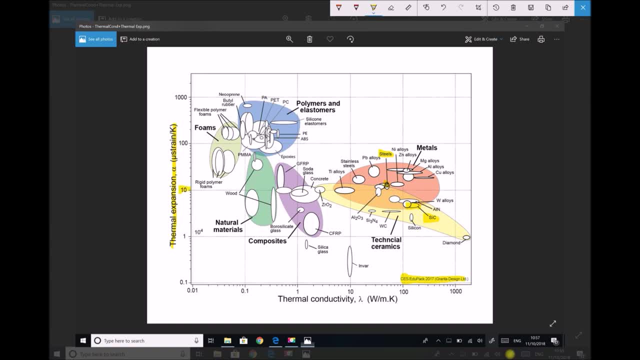 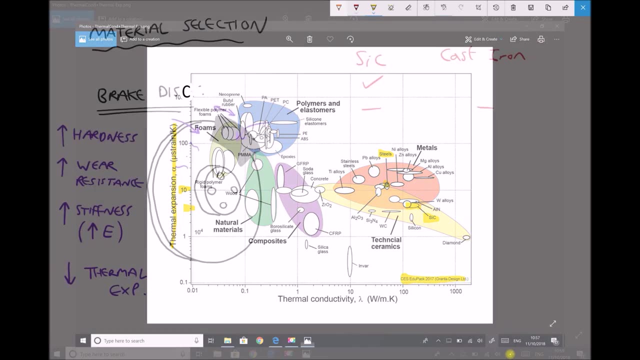 of thermal expansion of around 10, whereas our silicon carbide has a coefficient of thermal expansion of around 4.. So, once again, the silicon carbide far outperforms the cast iron. So let's summarize: We've already established that silicon carbide is the harder of the two materials. but